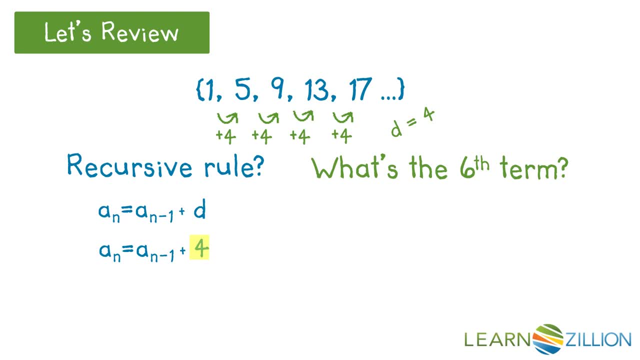 Using this rule, what's the sixth term for the sequence? Since we're trying to find the sixth term, we're going to use the recursive rule to find the next term. n must equal 6.. So we have a sub 6 equals a sub 5 plus 4.. 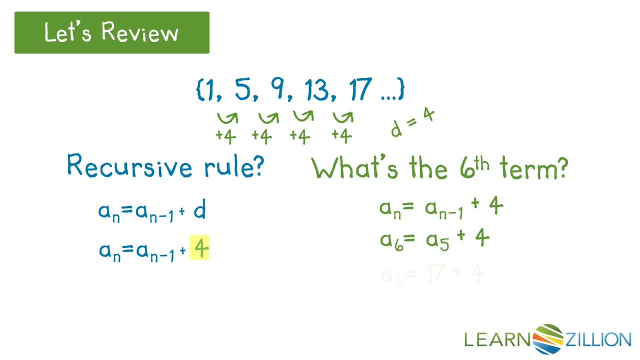 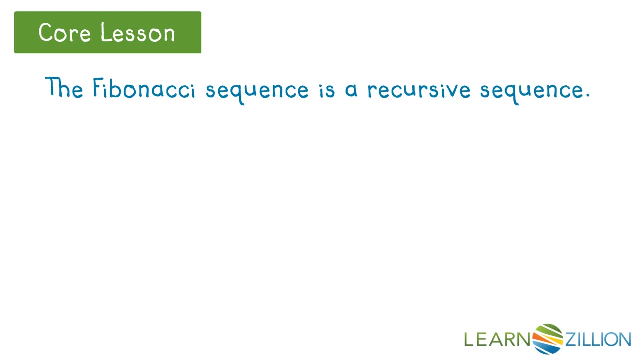 A sub 5 represents the fifth term, and the fifth term is 17.. So we have a sub 6 equals 17 plus 4.. A sub 6 equals 21.. The Fibonacci sequence is a recursive sequence, because the previous two terms are added together. 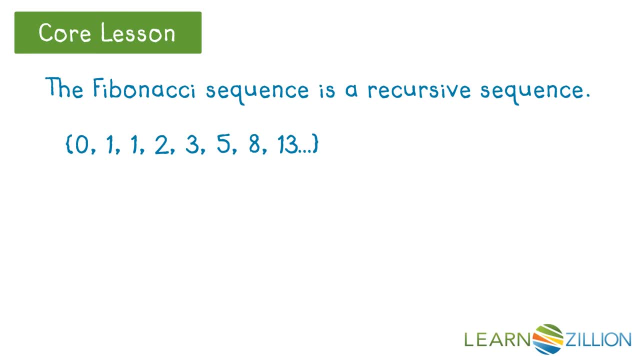 to find the next term, Let's take a look at the Fibonacci equation. When 0 and 1, the first two terms are added together, we get 1,, which is the third term. When 1 and 1, the second and third terms are added together, we get 2,, which is the 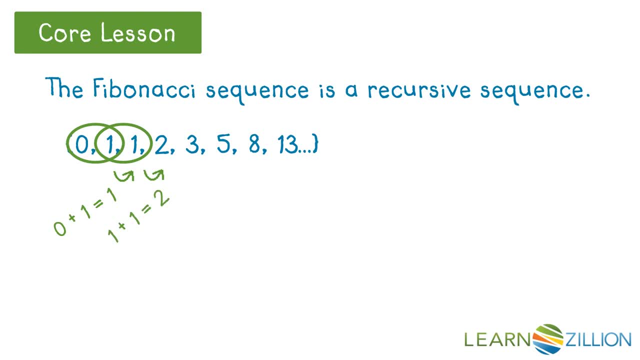 fourth term In the Fibonacci sequence. for any terms greater than 2, the previous two terms are added together to find the next term. This can be represented with the rule: a sub n equals a sub n minus, 1 plus a sub n minus. 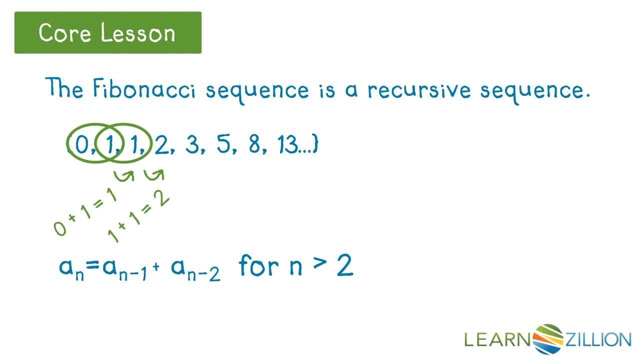 2, 4n is greater than 2.. But let's test out this rule to make sure it does work. We know the eighth term in the Fibonacci sequence is 13,, so let's use n equals 8.. We get a sub 8 equals a sub 8 minus 1, plus a sub 8 minus 2, which gives us a sub 8 equals. 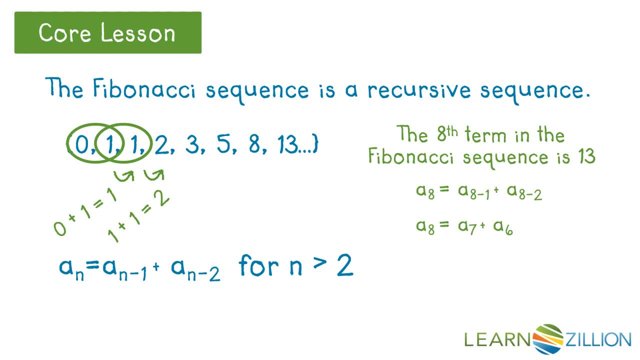 a sub 7 plus a sub 6.. The seventh term is 8, and the sixth term is 5.. So now we have 13 equals 8 plus 5.. So now we have a sub 8 equals a sub 8 minus 1 plus a sub 8 minus 2,, which gives us a sub. 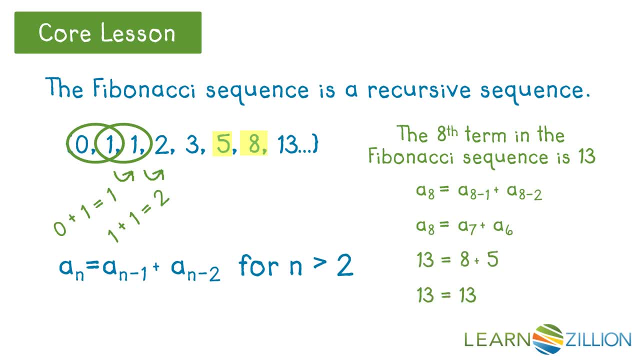 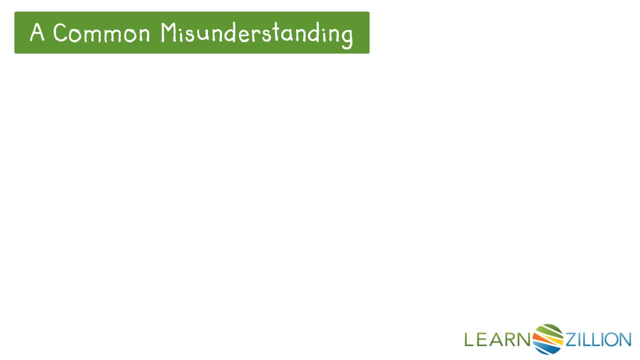 8 equals a sub 7 plus a sub 6.. Since we know, 8 plus 5 is 13,, we have a true statement. So this recursive rule does represent the Fibonacci sequence. It's a common misunderstanding to think that the Fibonacci sequence follows the general. 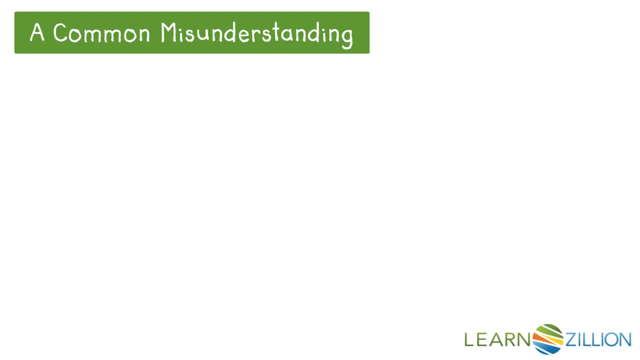 recursive rule, but the Fibonacci sequence does not follow the general recursive rule. Let's take a look. To move from the third term, which is 1,, to the fourth term, which is 2,, we add 1.. To move from the fourth term to the fifth term, we add 1.. 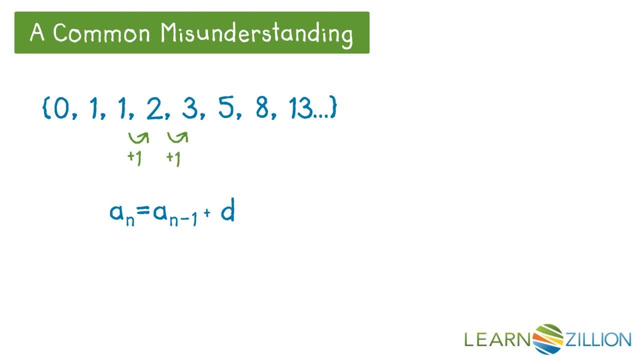 To move from the fourth term to the fifth term: we add 1.. We add 1.. term: we also add 1.. So it's easy to think that there's a common difference and that this common difference is 1.. So if we assume that D is 1 and we substitute that value into 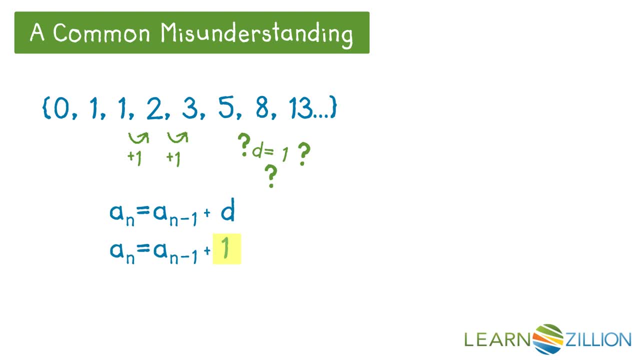 the general recursive rule. we have a sub n equals a sub n minus 1 plus 1.. But does this rule work with the Fibonacci sequence? The sixth term of the Fibonacci sequence is 5.. So let's test out the rule with n equals 6.. We have a sub 6 equals a sub 6 minus 1. 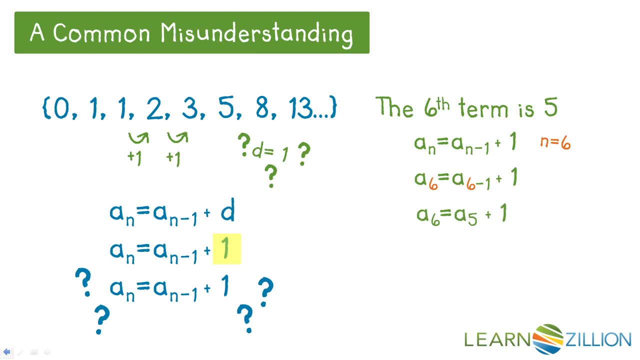 plus 1, which is a sub 6, equals a sub 5 plus 1.. The value of the sixth term is 5 and the value of the fifth term is 3.. So now we have 5 equals 3 plus 1.. But 3 plus 1 is 4 and 5. 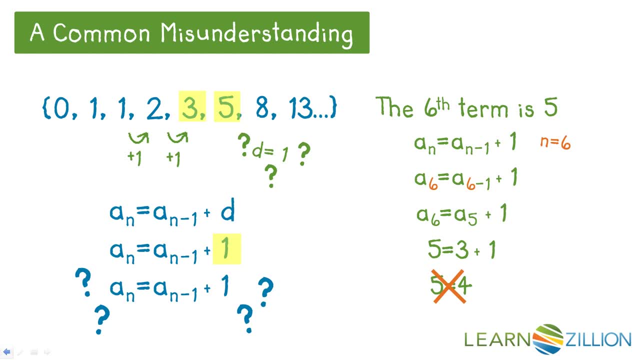 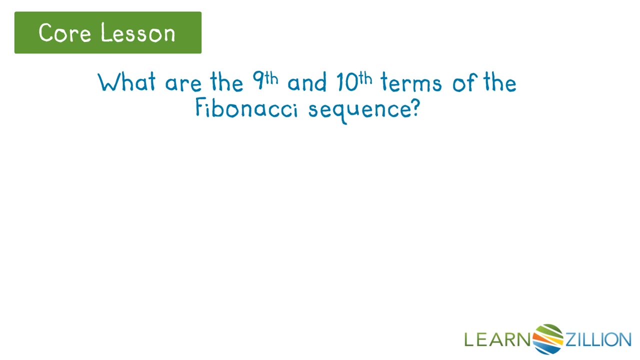 doesn't equal 4.. So we know that this is a false statement. The Fibonacci sequence does not have a common difference And it does not follow the general recursive rule. What are the ninth and tenth terms of the Fibonacci sequence? To find the ninth term, we will use: a sub 9 equals a sub 8 plus. 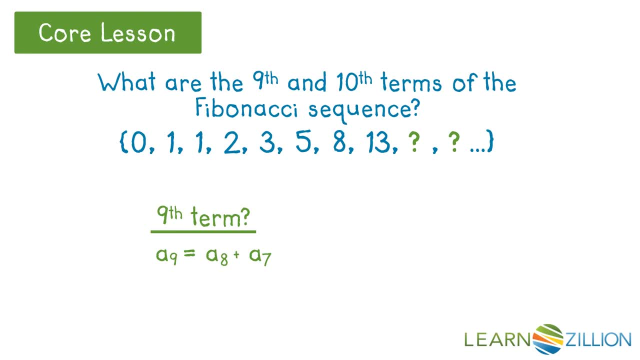 a sub 7.. a sub 8 is 13 and a sub 7 is 8.. So a sub 9 is 13 plus 8.. a sub 9 is 21.. The ninth term of the Fibonacci sequence is 21.. 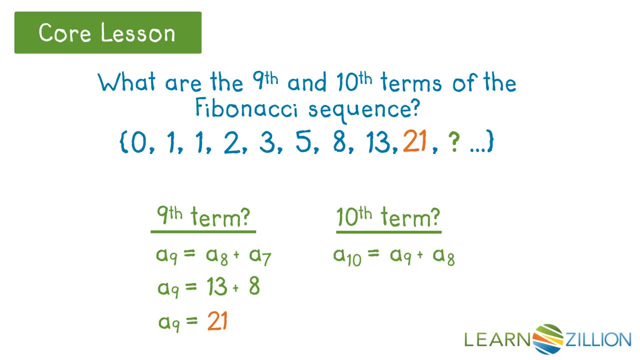 What's the tenth term? To find it, we will use: a sub 10 equals a sub 9 plus a sub 8.. We just found out that a sub 9 is 21 and a sub 8 is 13.. So a sub 10 is 21 plus 13.. a sub: 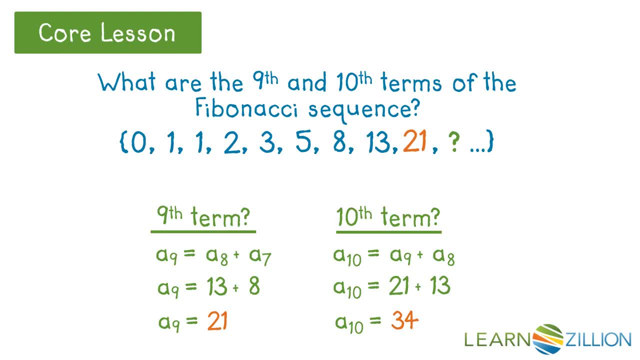 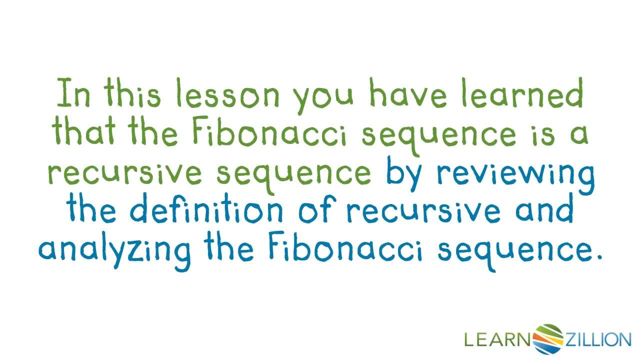 10 equals 34.. The tenth term in the Fibonacci sequence is 34.. The Fibonacci sequence is a recursive sequence because for terms greater than 2, the previous two terms are added together to find the next term. In this lesson you have learned that the Fibonacci sequence is a recursive sequence. 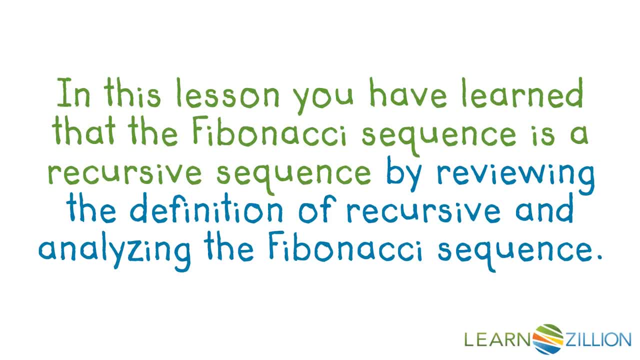 by reviewing the definition of recursive and analyzing the Fibonacci sequence.